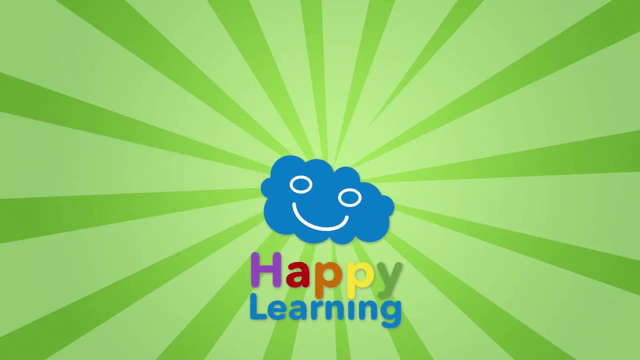 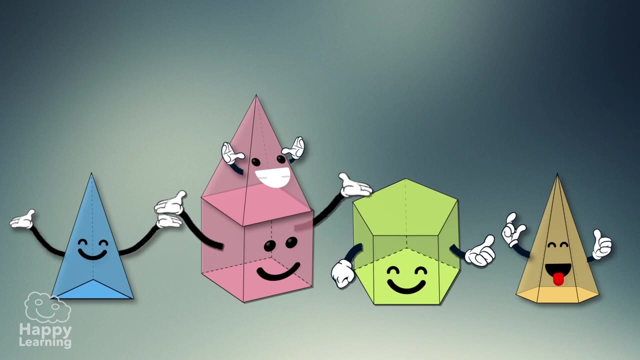 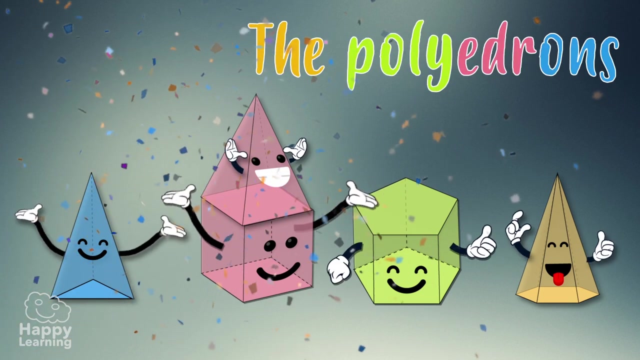 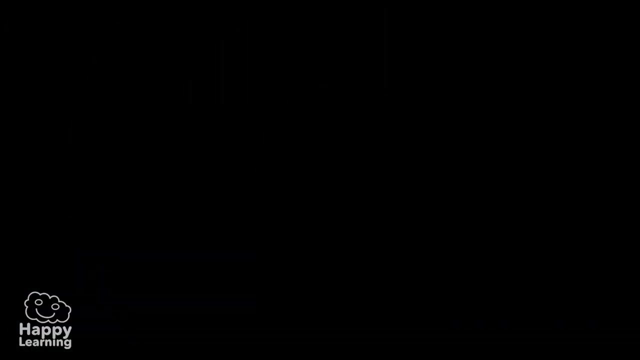 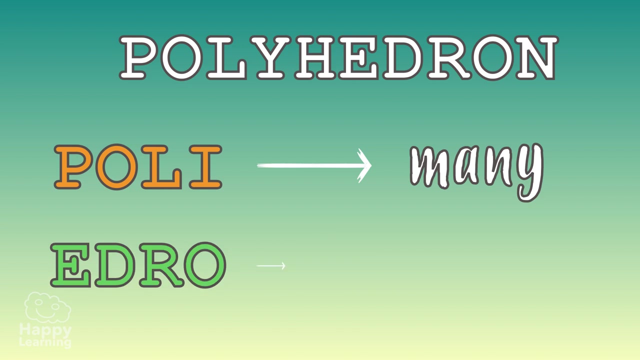 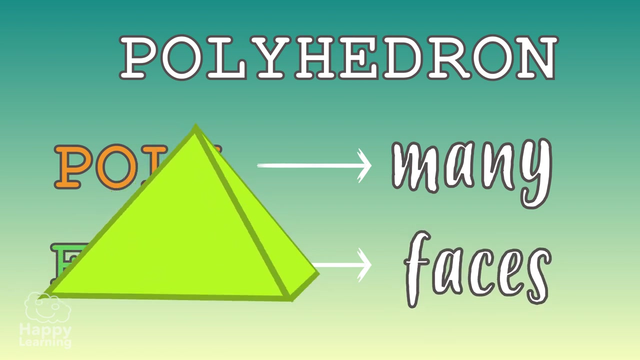 Hello friends, welcome to a new happy learning video. Today we are going to learn about the polyhedrons. The word polyhedron comes from Latin poly, meaning many, and edro faces, so its name tells us that polyhedrons have many faces. 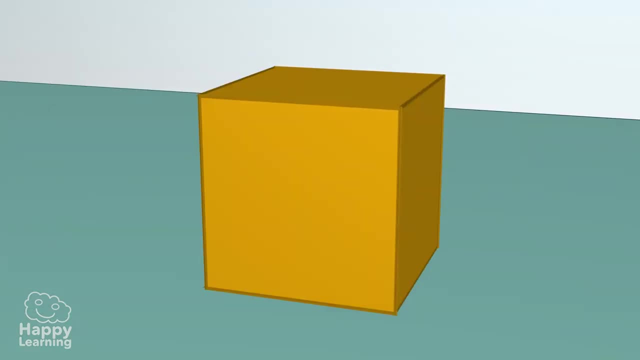 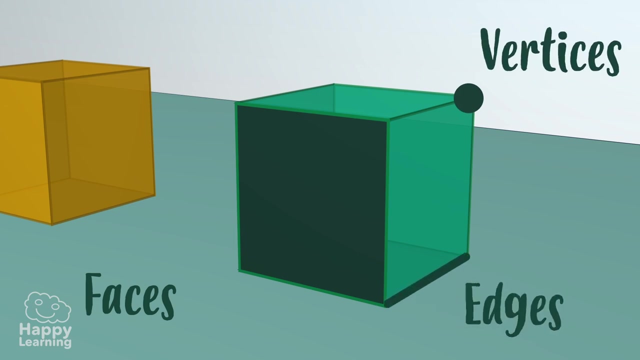 Polyhedrons are geometric bodies formed by several polygons. They have volume, that is, they occupy space in three dimensions: width, length and height. A very important thing that you also have to know about polyhedrons is that they are formed by three different elements: faces, vertices and edges. 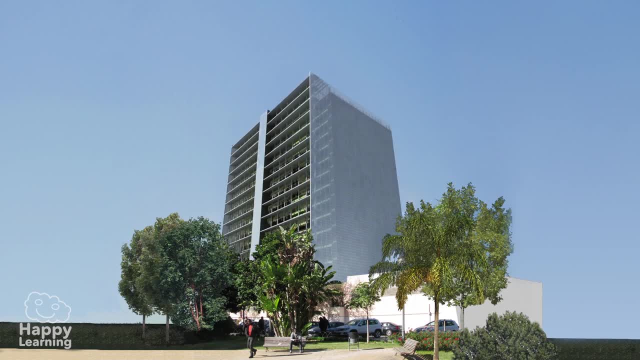 Observe this building and we will go discovering the three elements. As you can see, this building is a polyhedron formed by quadrilaterals, which are polygons with four sides. Well, faces are the polygons that make up the polyhedron. 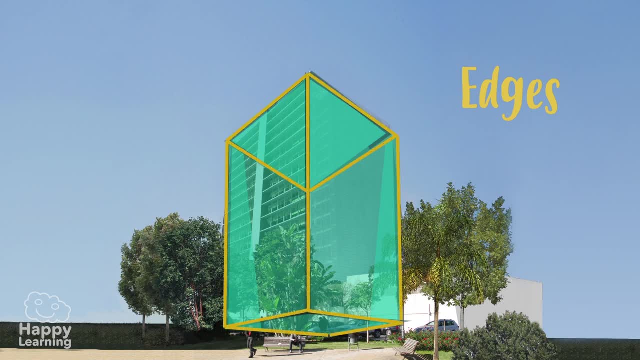 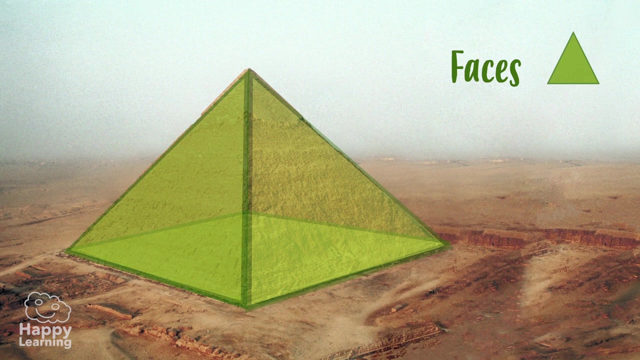 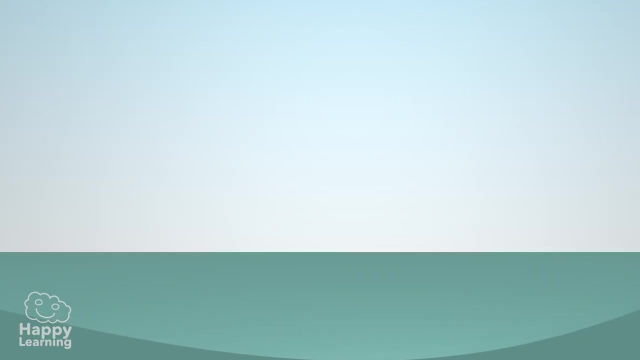 The edges are the sides of the faces and the vertices are the points where three or more faces meet. Now observe this pyramid of Egypt and we will discover its faces, vertices and edges. Easy, eh. Polyhedrons can be classified in many ways, but there are two types that we have to know. 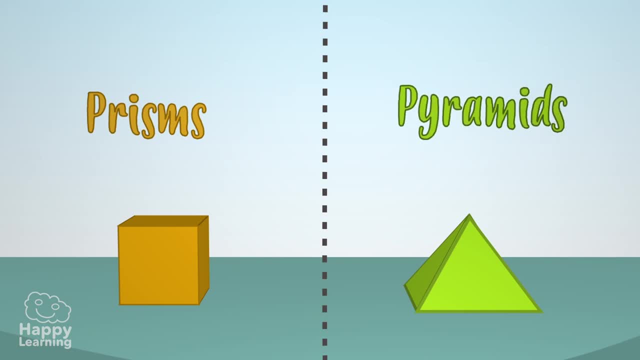 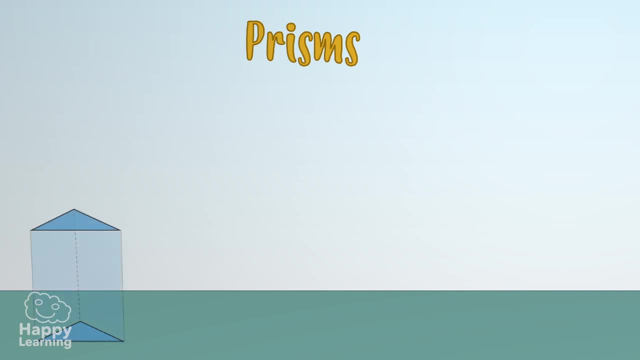 They are the prisms and the pyramids. The prisms have two polygonal bases and the number of sides of the bases are called triangular prism if it has three sides, quadrangular prism if it has four sides, pentagonal if it has five, hexagonal if it has six, and so on. to infer that the prisms are the same.